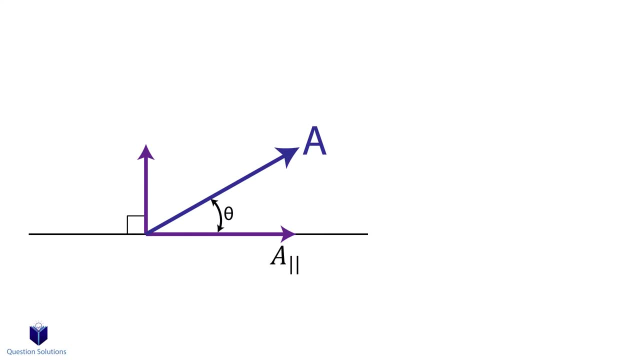 and it's referred to as the projection of a force. To find it, all we need to do is take the dot product between the force expressed in Cartesian form and the univector of the axis or the side where the projection is supposed to be. If we need to find the perpendicular component, 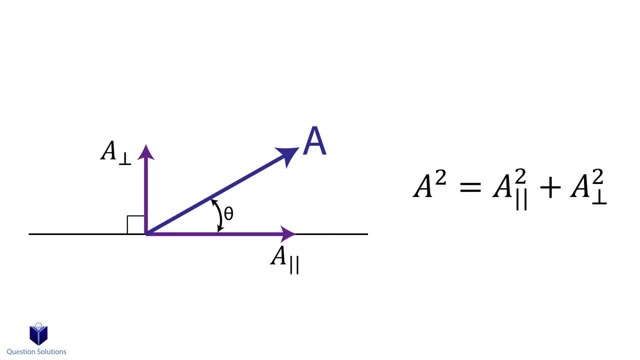 then we can use this equation to do it. It's just the Pythagorean theorem Here. this is the magnitude of the force. This is the magnitude of the force. This is the parallel component And this is the perpendicular component. This will become much more clear with examples, but to do so you should be able to express. 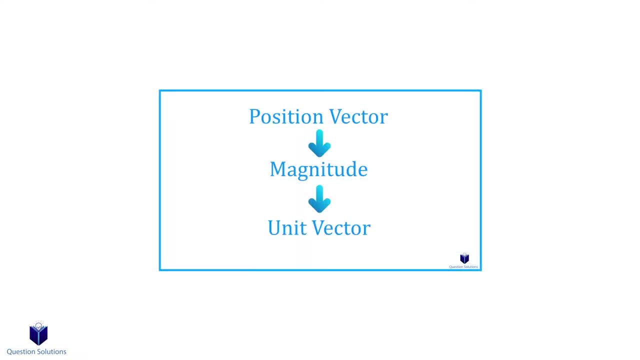 forces in Cartesian form and be able to write position vectors along with unit vectors. In the previous video I go through this step by step, so if you need a refresh or you forgot, please check the description. Now let's move on to some examples and see. 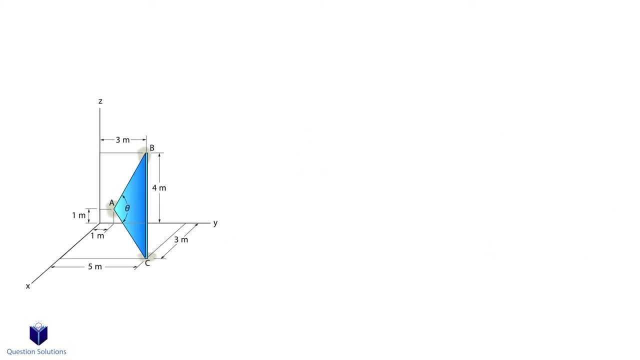 how we can find angles, projections and more. Let's take a look at this question, where all we need to do is figure out the angle between the two sides of the triangular plate. We're going to do it using the dot product, So let's write down the equation to figure out an. 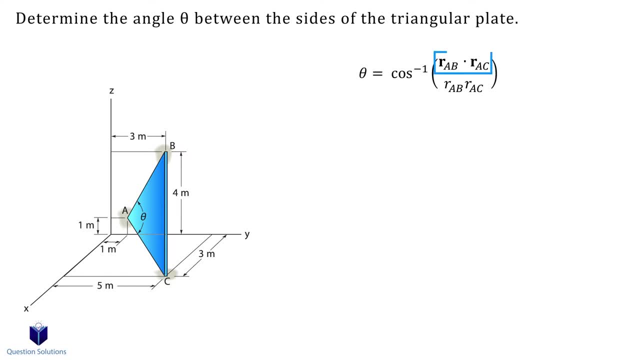 angle. So first we need two position vectors for the two sides of the triangle, one from A to B and one from A to C. Let's write down the locations of points A, B and C. Now we can write our position vector. Let's simplify Next: a position vector from A to B. 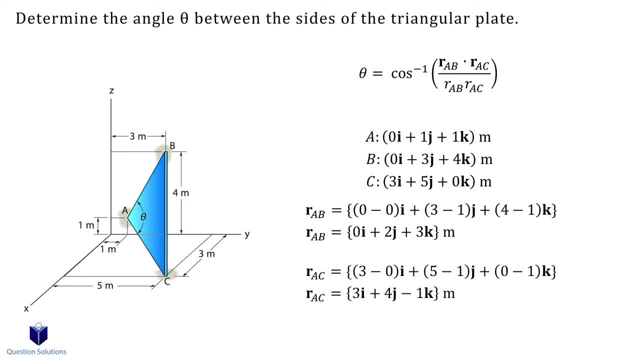 from A to C. Now we need to find the magnitude of these position vectors. Next we will take the dot product between the two position vectors. So all we're doing is multiplying i components by i components, j components by j components and k components by k components. The result is a scalar value. Now all that is left is to 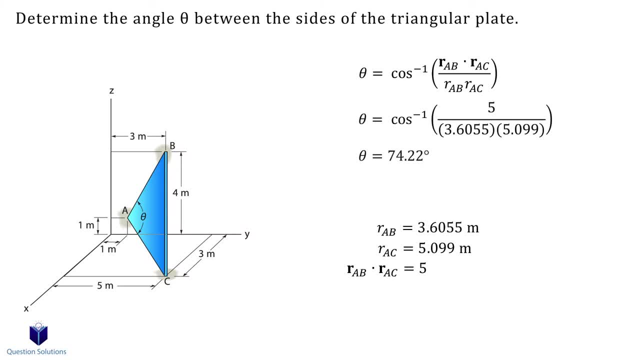 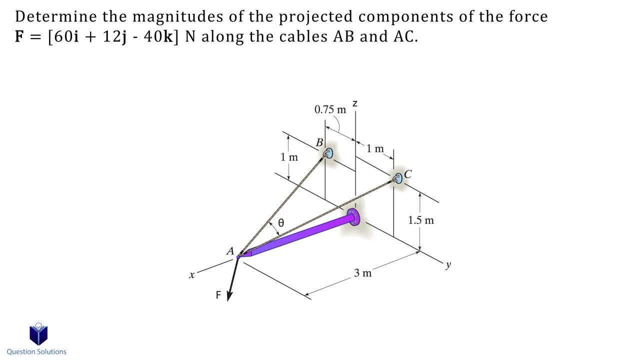 plug everything into our equation. Solving gives us our answer. Let's take a look at this question. So we have a question involving projections. We need to figure out the magnitudes of the projected components of the force along cables AB and AC When we have questions asking for 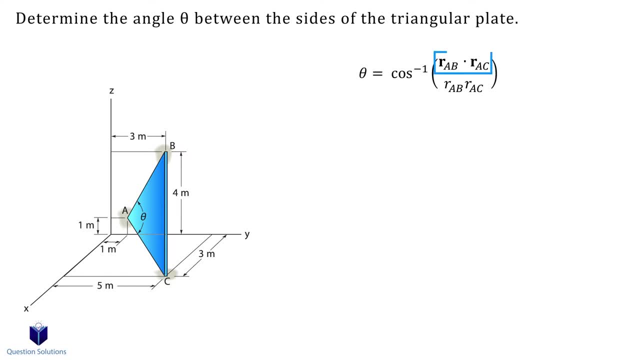 angle. So first we need two position vectors for the two sides of the triangle, one from A to B and one from A to C. Let's write down the locations of points A, B and C. Now we can write our position vector. Let's simplify Next: a position vector from A to B. 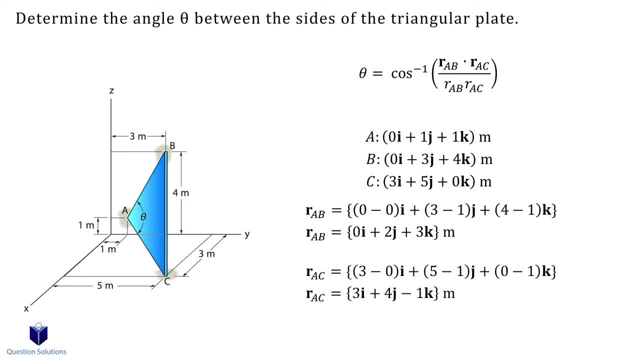 from A to C. Now we need to find the magnitude of these position vectors. Next we will take the dot product between the two position vectors. So all we're doing is multiplying i components by i components, j components by j components and k components by k components. The result is a scalar value. Now all that is left is to 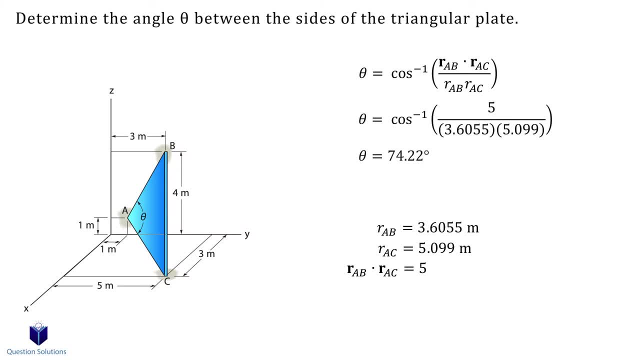 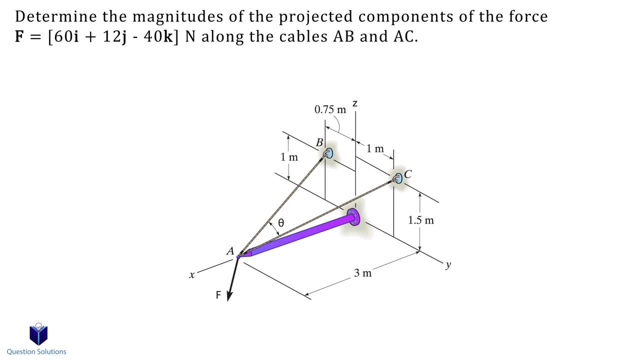 plug everything into our equation. Solving gives us our answer. Let's take a look at this question. So we have a question involving projections. We need to figure out the magnitudes of the projected components of the force along cables AB and AC When we have questions asking for 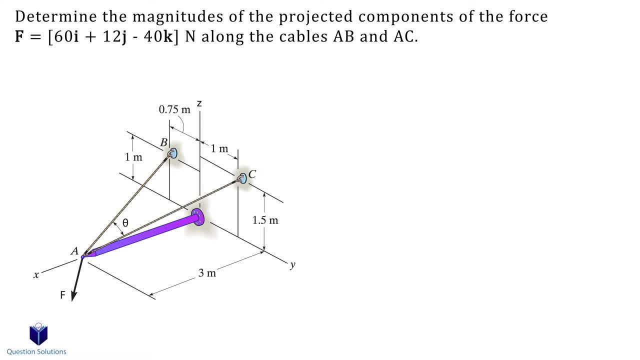 projections, we need to find unit vectors. So in this problem we need a unit vector for cable AB and cable AC. So let's start by writing down the locations of each point. So we have points A, B and C. Next we need a position vector from A to B and A to C. 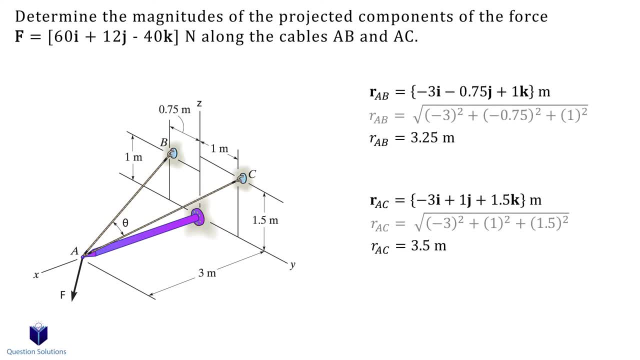 Now we can find the magnitude, Okay. so finally we can divide each component in our position vector by the magnitude and we get our unit vectors. We're now ready to do the dot product First, the projection of force F onto cable AB. For that, all we need to do is take the dot product. 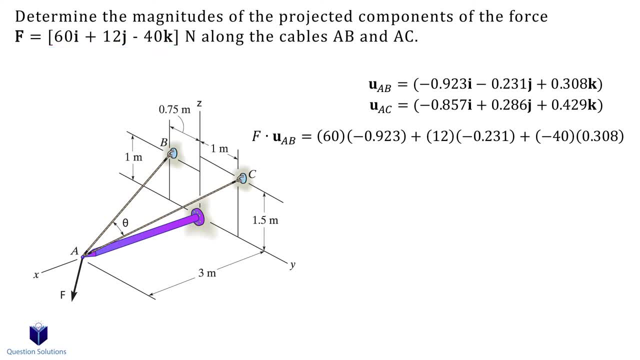 between force F and the unit vector AB. Remember force F has to be expressed in Cartesian form and since the question already gives it in Cartesian form, we can just take the dot product. Since we're asked for the magnitude, remember it'll be positive. The negative sign means that 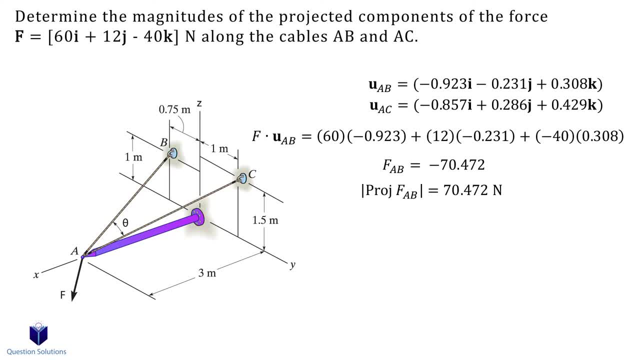 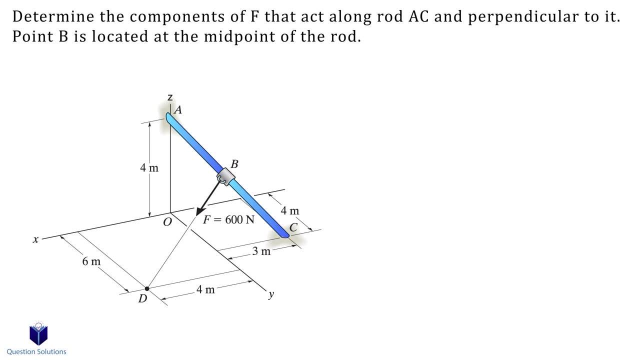 our component points in the opposite direction to the unit vector. Next, the projection of force F onto cable AC. Those are our answers. Let's take a look at this problem, where we need to find the projected component of the 600 Newton force along rod AC, Unlike 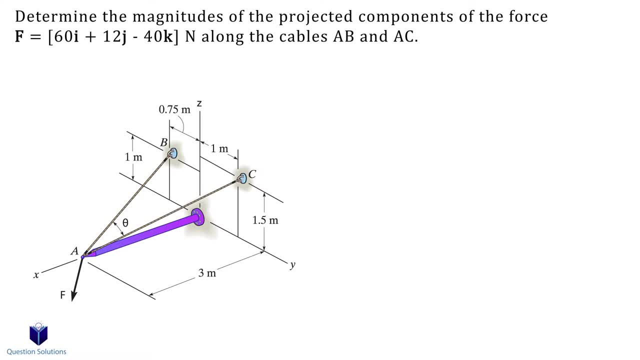 projections, we need to find unit vectors. So in this problem we need a unit vector for cable AB and cable AC. So let's start by writing down the locations of each point. So we have points A, B and C. Next we need a position vector from A to B and A to C. 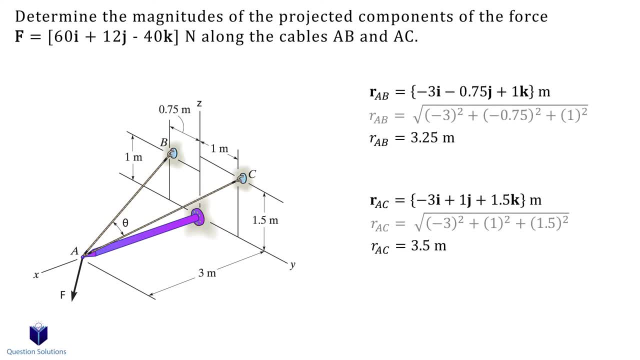 We can find the magnitude. Finally, we can divide each component in our position vector by the magnitude and we get our unit vectors. We're now ready to do the dot product First, the projection of force F onto cable AB. For that, all we need to do is take the dot product. 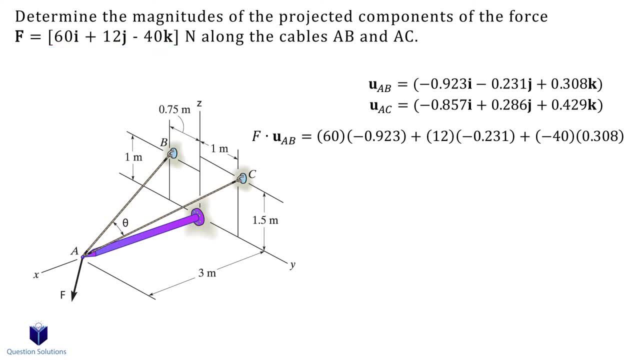 between force F and the unit vector AB. Remember force F has to be expressed in Cartesian form and since the question already gives it in Cartesian form, we can just take the dot product. Since we're asked for the magnitude, remember it'll be positive. The negative sign means that 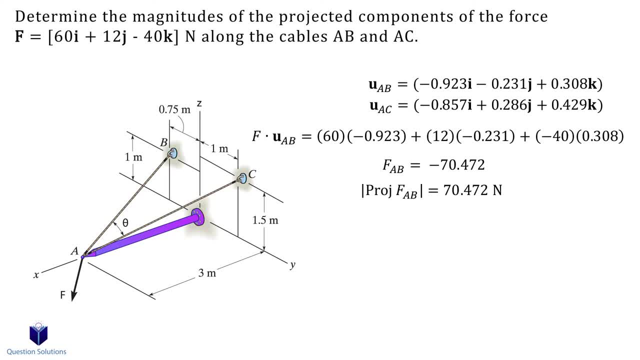 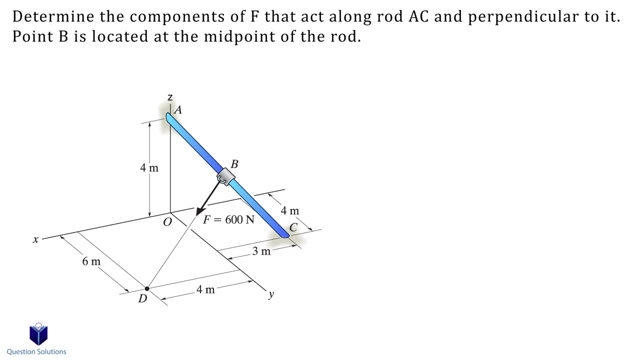 our component points in the opposite direction to the unit vector. Next, the projection of force F onto cable AC. Those are our answers. Let's take a look at this problem, where we need to find the projected component of the 600 Newton force along rod AC, Unlike 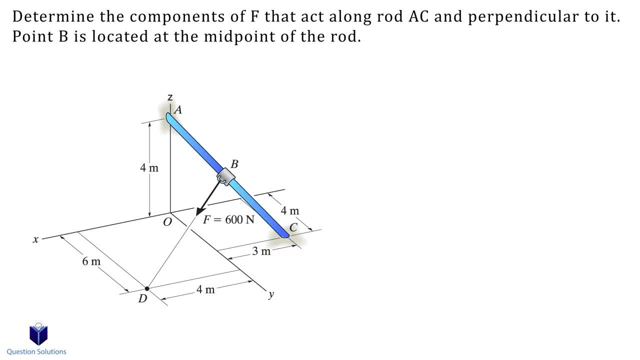 the previous question. our force isn't given in Cartesian form, so we need to express it as such. After that we need a unit vector for rod AC. So to do all this, we first need to write down the locations of all the points of interest. First, point A. Next we need to figure out point B. 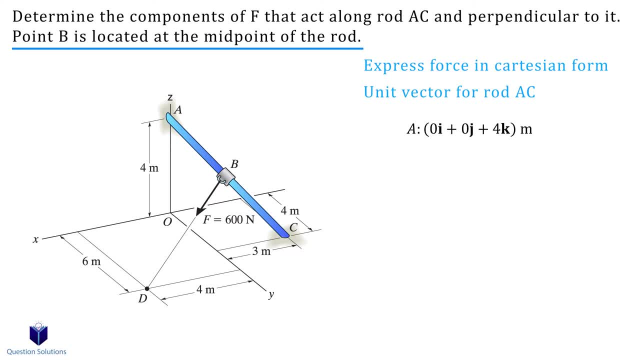 The question says point B is at the midpoint of rod AC. So the x component would be 1.5 meters. in the negative x direction, The y component would be 2 meters and the z component would also be 2 meters. We're just dividing the distances by 2.. 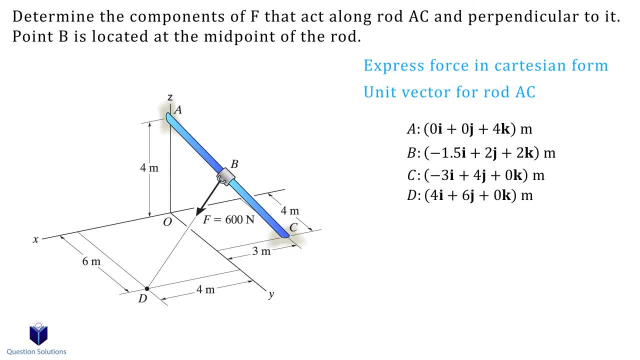 Next we have point C and D. To express the 600 Newton force in Cartesian form, we need a position vector from B to D. Now we need the magnitude of this vector. Next step is to divide each component in our position vector by the magnitude. 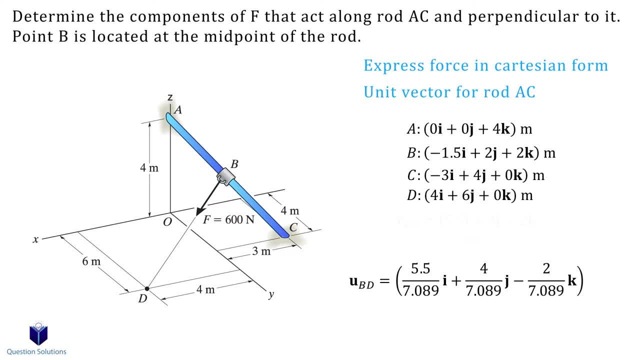 which gives us our unit vector. We just multiply the magnitude of the force by the unit vector and that is our force expressed in Cartesian form. Now we need a unit vector for rod AC. The process is pretty much the same: First a position vector from A to C, Now the magnitude And lastly,